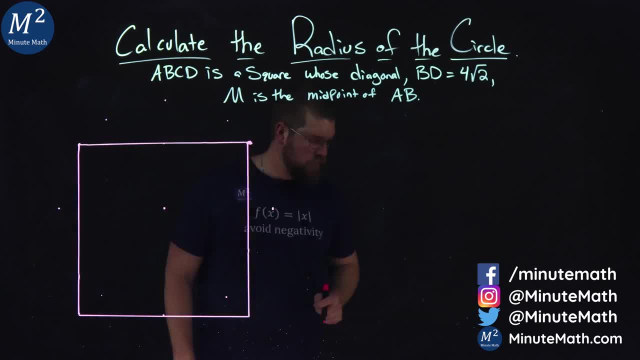 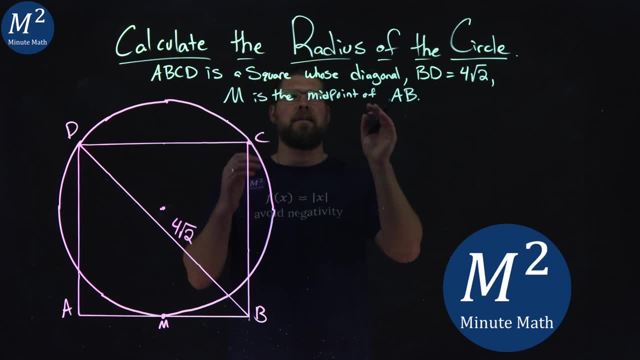 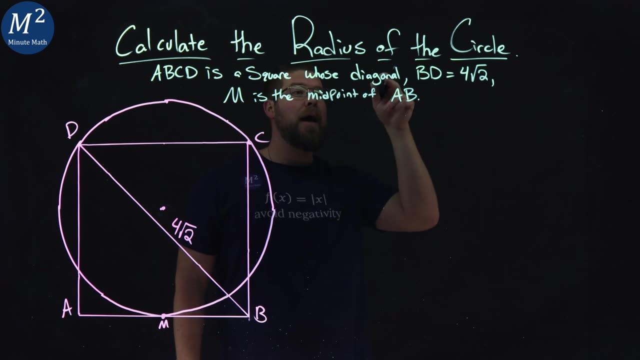 Hi, I'm Sean Gannon and this is Minute Math and we've got to calculate the radius of the circle. We're given some key information. first, ABCD is a square important whose diagonal BD is equal to four square root of two M is the midpoint of- excuse me- line segment AB. What we want to do, 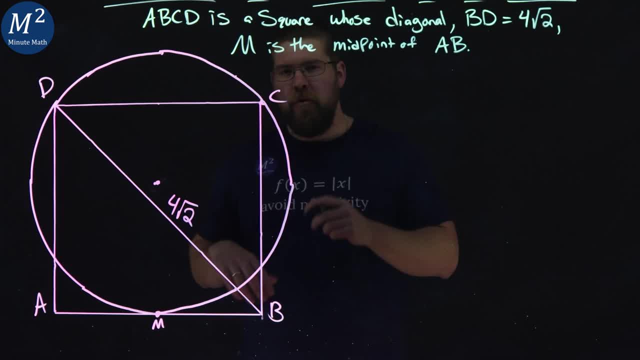 again is find the radius of the circle. Now a few clues here. Let's go fill in what we know. Since ABCD is a square, we know we got some right angles going on here. All right, not too bad, We can do that. Now they say AB has midpoint M, meaning these two lengths are going to be. 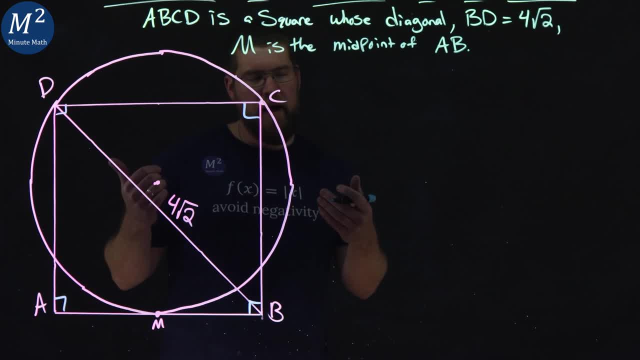 congruent, So we can find the overall length of AB. We can break that in half. Now let's go look at this diagonal: DBBD, four square root of two. Okay, that's our hypotenuse. if we see a right triangle Triangle, let's call it DCB. 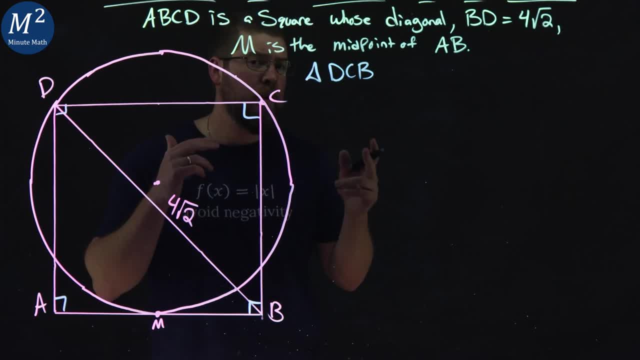 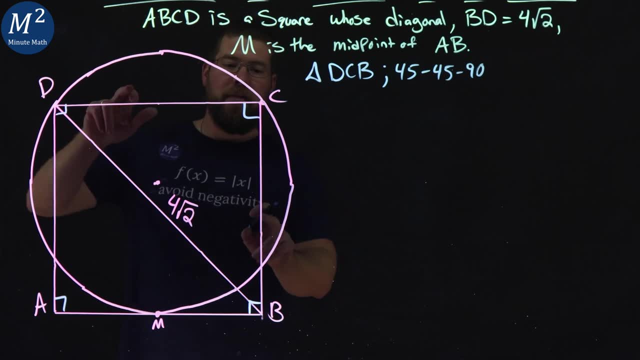 DCB is a special right triangle. It's actually a 45,, 45, 90.. How do I know that We got a right angle right here and these two side lengths are the same? because we got a square right there, meaning these two sides are going to square, same side length. We know that it's. 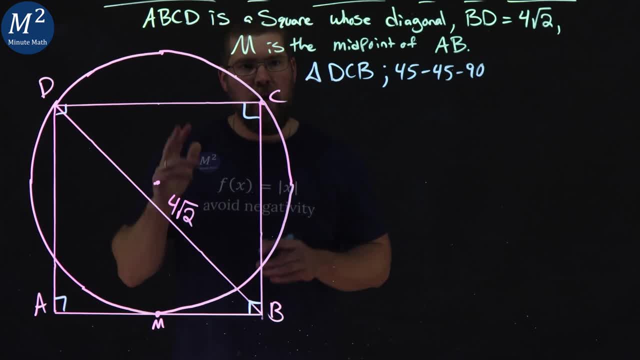 going to cut it right here in half, and each one of these will be 45.. So this triangle has the form of a one one square root of two. form meaning we can extrapolate that with our hypotenuse of four square root two, We can figure out what the length of well. 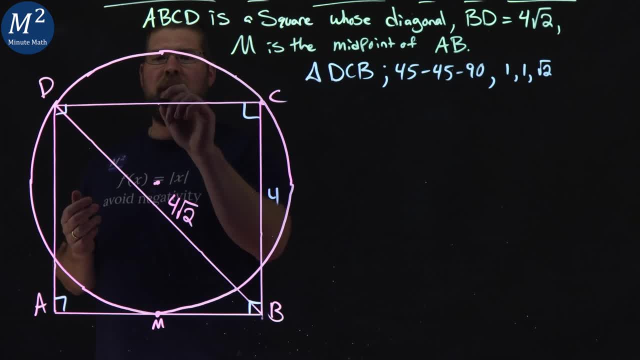 every side. length: that's going to be four here. Now. we also could have done that with Pythagorean theorem if you wanted to as well, but I just did it like that. All right, Now. with that that means length: AM is going to be a two, and this length here is a two because remember. 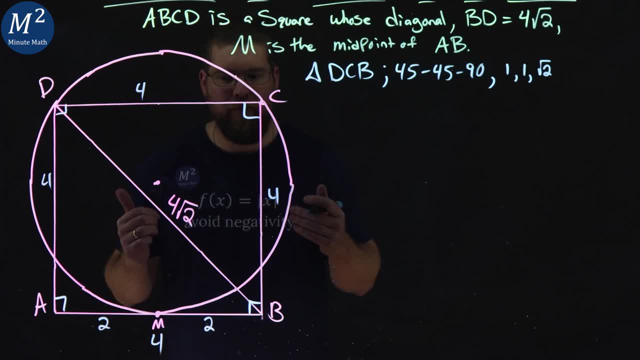 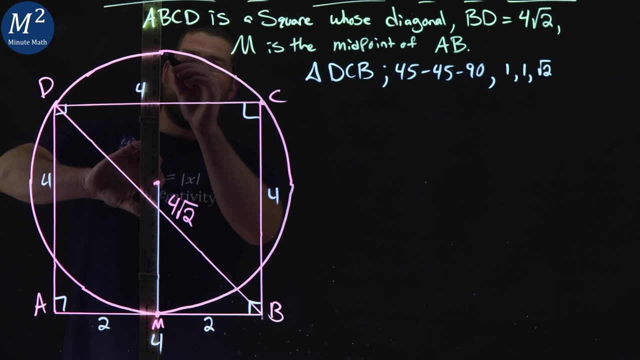 M splits line segment AB in half. All this goody-goody information. Now let's go draw a radius here from the center of the circle down to M, and let's keep going up as well. So if I can draw this, here, we got a radius. let's call that here down to M, all the way up to the top. 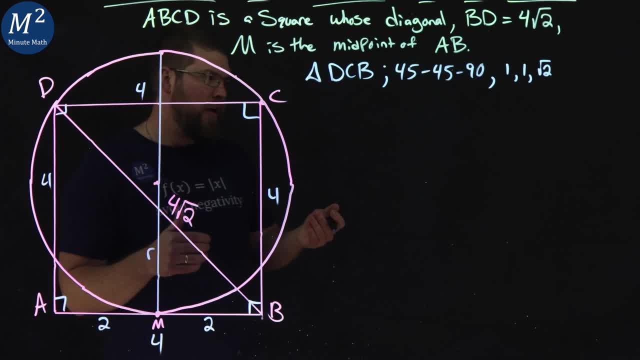 All right, Let's call that R here. and what do we know? If a radius is tangent to the circle at that point here, that line tangent to the circle, it's going to be a right angle. Got that Same thing here We're going up. We got a radius of R from that circle. point right there Again. 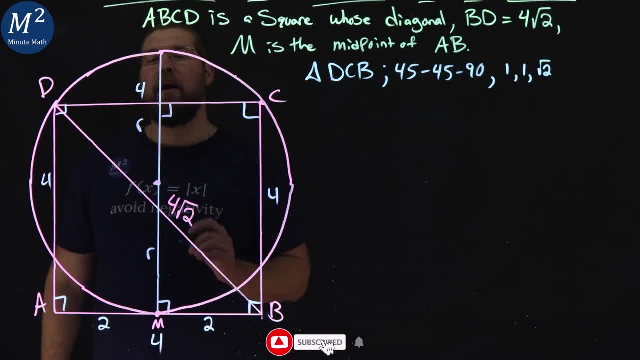 if it's perpendicular here at the base, it must be perpendicular up here. All right, Now here comes the tricky part. What is the length here of this? to this, What did I label this point? Did I label it? I called it F and E. So we have: let's call this point here F and this point here E. 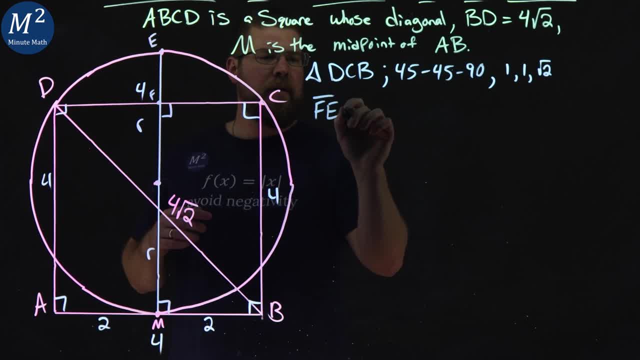 What is the length of F- E? How can we find that? Well, we have the overall length of the whole circle, which is going to be 2R, right, R being the radius, 2R minus the length of the square to that point here, right F to M, which is going to be 4,. 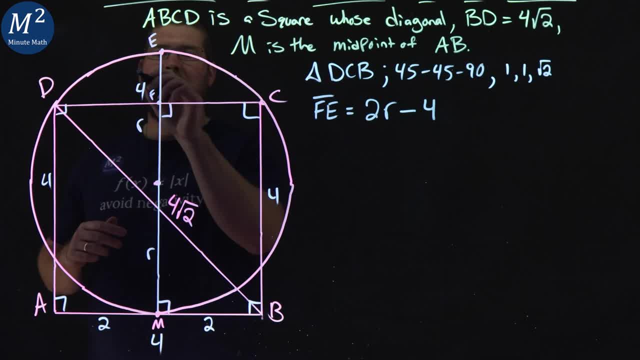 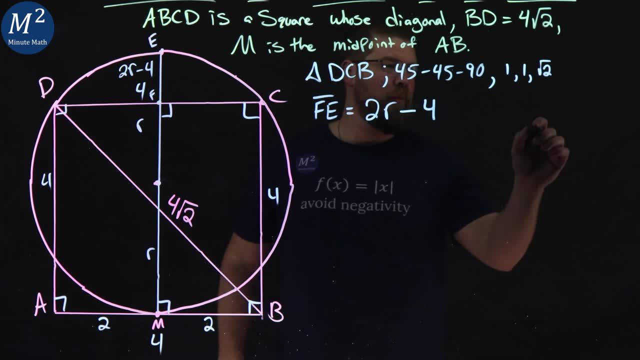 right there. So F? E has a length of a 2R minus a 4.. All right, Now this is the tricky part. Here's called the intersecting chords theorem. We draw a circle here. Let's get a little image of. 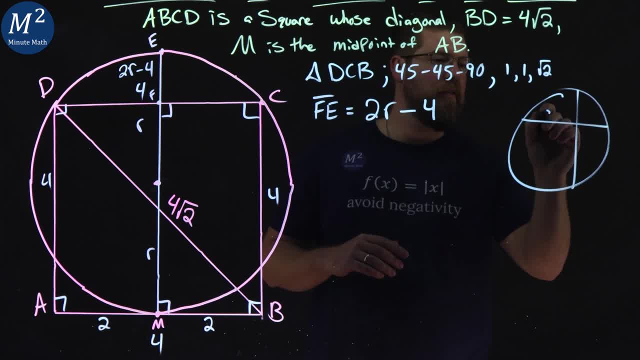 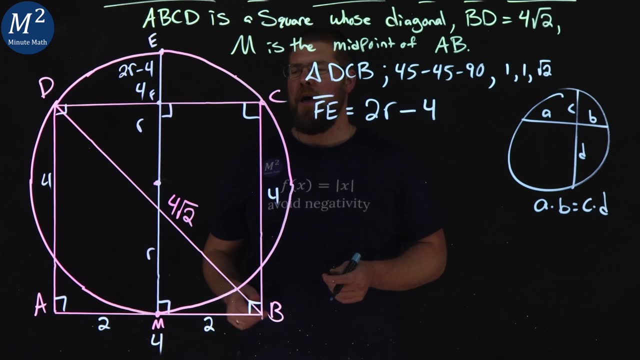 it. We have two chords that intersect. Let's call this side. We have length AB and CD. They tell us if we have two intersecting chords. what we can write here is: A times B is equal to C times D. intersecting chords theorem. How does it apply here? Well, 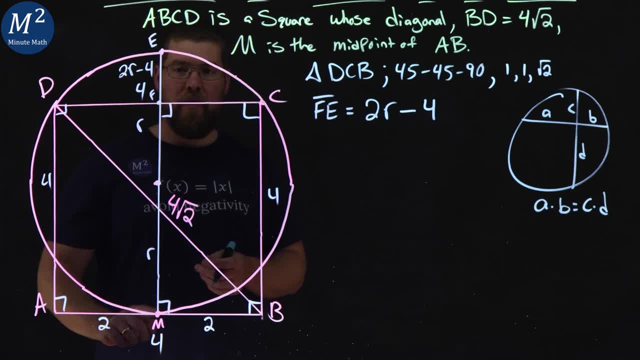 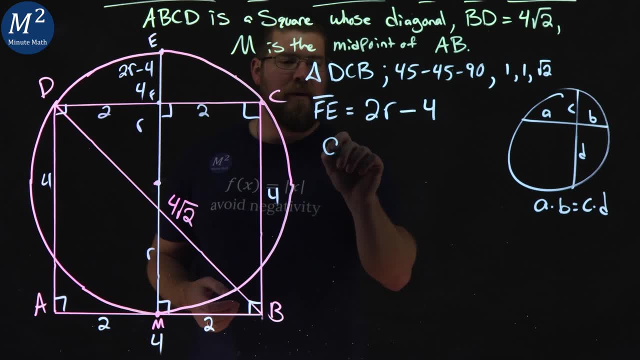 I have one chord going on. I can see this big line AM, and we're intersecting with the C board of these lengths, Same here, 2, 2.. So if I rewrite this to be AB equals a CD, multiply it out A and. B, I would call it 2R. So if I rewrite this to be AB equals a CD, multiply it out A and B, I would call it 2R. So if I rewrite this to be AB equals a CD, multiply it out A and B, I would call it 2R. 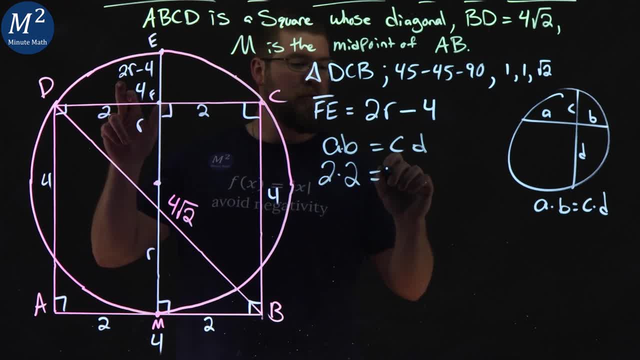 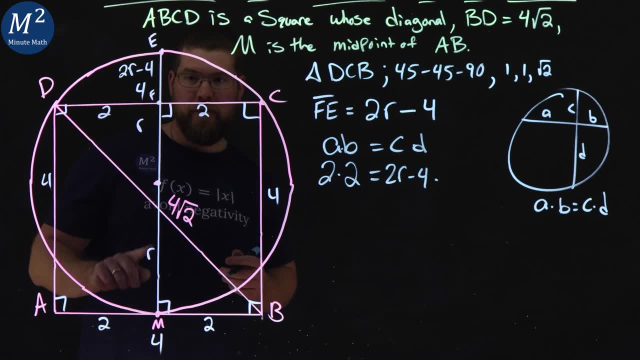 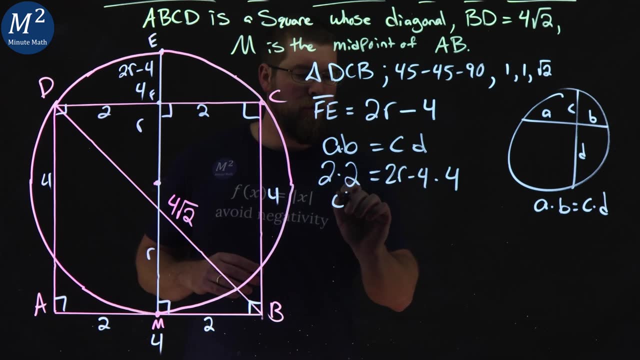 2 times 2.. And CD, we have 2R minus 4 times D, this length here, D, which is the length from F to M, which is F4.. From there we want to well solve for R. That's what we're looking for. We got 4.